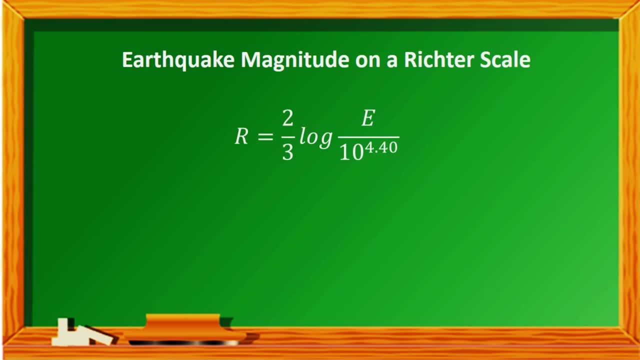 The magnitude R of an earthquake is given by. R equals two-third log of E over 10 raised to the power of 4.40, where E is the energy released by the earthquake in joules and E is the energy released by the earthquake in joules. 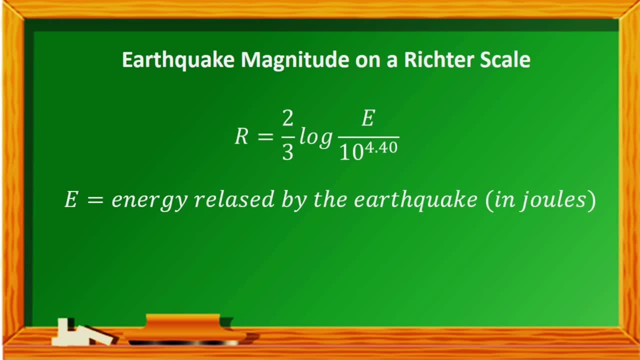 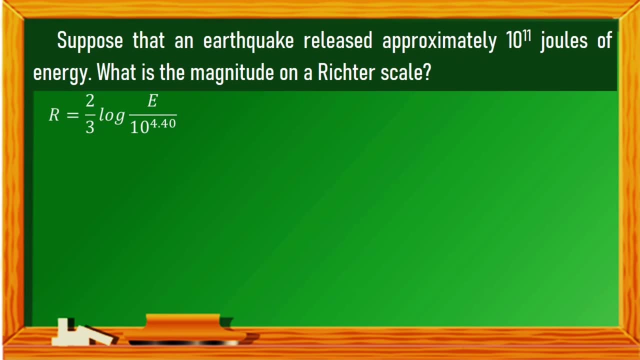 And the quantity, 10 raised to the power of 4.40, is the energy released by a very small reference earthquake Sample problem. suppose that an earthquake released approximately 10, raised to the power of 11 joules of energy, What is the magnitude on a Richter scale? 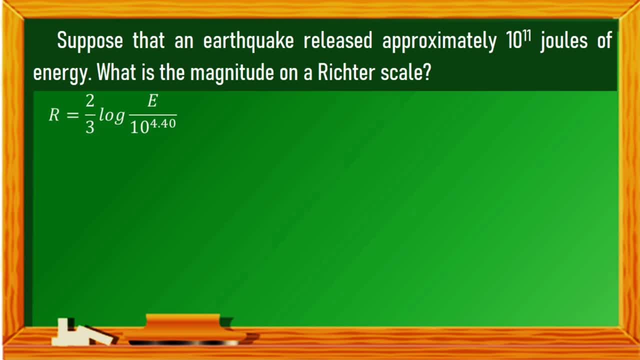 We will use the formula of the magnitude R of an earthquake, Since the energy released by the earthquake is 10 raised to the power of 4.40, and the magnitude of the earthquake is 10 raised to the power of 11 joules of energy. 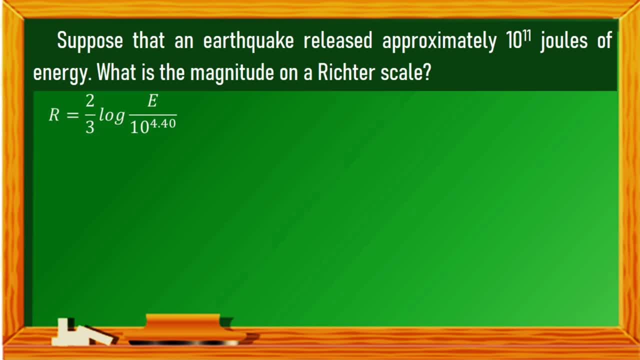 then let us substitute this to the formula. To solve this, let us apply one of the laws of exponents: quotient of powers. This states that in dividing two powers with the same basis, we subtract the exponents 11 minus 4.40 is 6.6.. 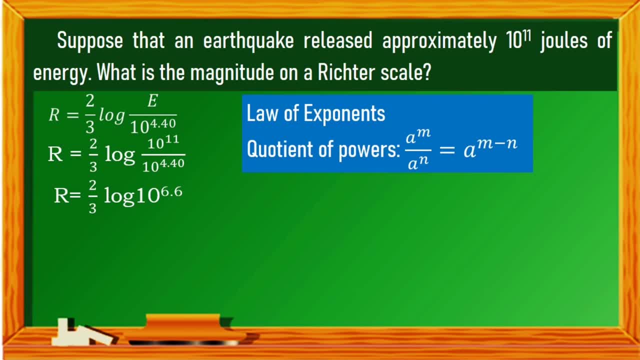